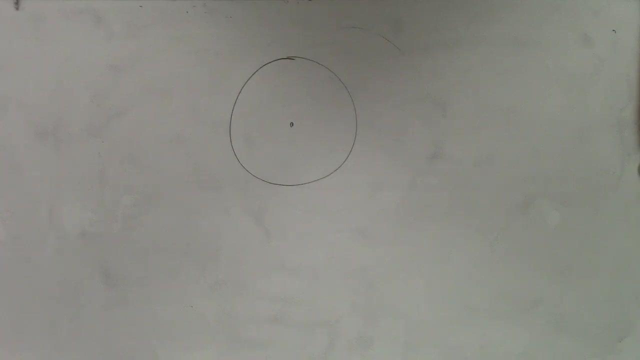 When, looking at this, what you guys missed last class period is what we call a central angle. A central angle was when you had an angle that had a vertex at the center. Okay, When you had a vertex at the center and you had two endpoints on there, which we'll call M and N. 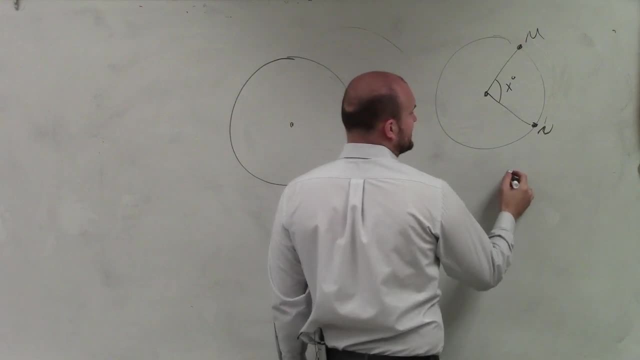 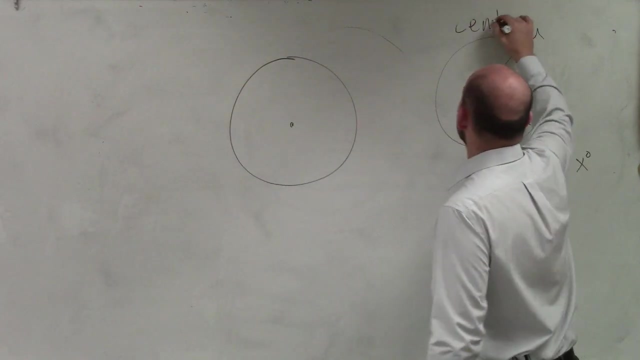 All right Now. what was important about this, Kaylee, was you noticed that the arc M N was equal to the measure of X degrees. This is what we called a central angle. All right, Kaylee, Thank you. 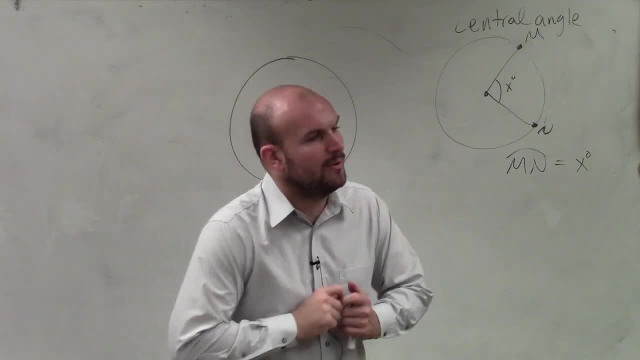 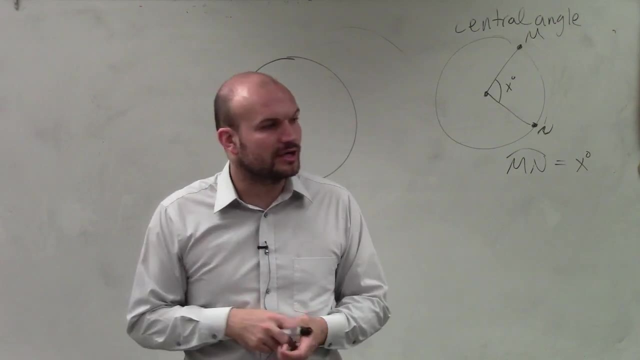 So now what we're going to be talking about is a new central angle, So I wanted to make sure, Kaylee, I went over that for the people that missed last class period, so then they can move from what is a central angle to now what we're going to call an inscribed angle. 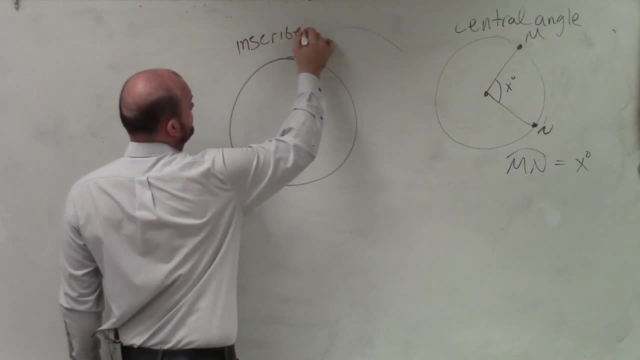 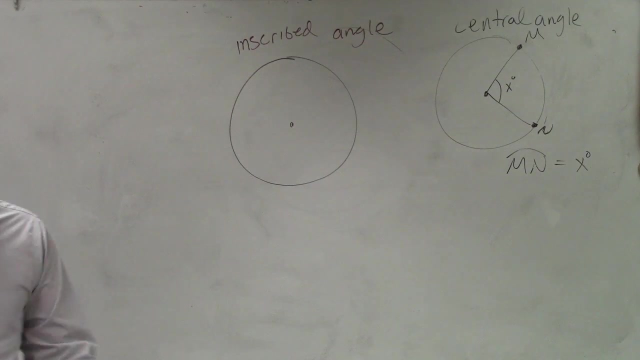 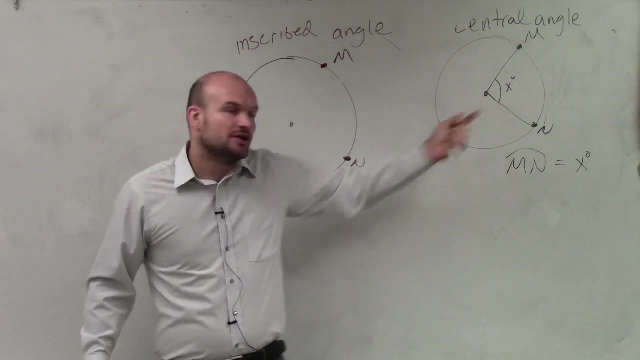 Yes. Now, when talking about an inscribed angle, the definition of an inscribed angle and how it differs from a central angle, is an inscribed angle is going to still have two endpoints on your circle. However, rather than having the vertex at the center, you're now going to have a vertex on the circle. 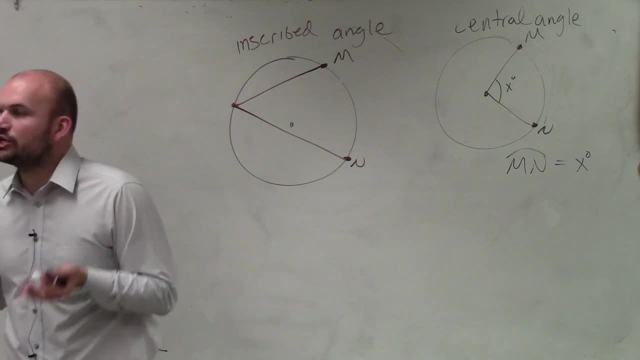 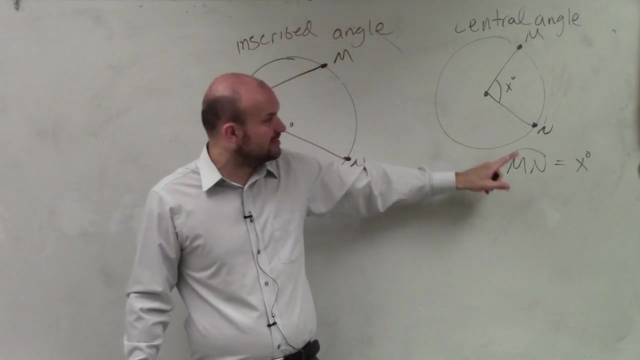 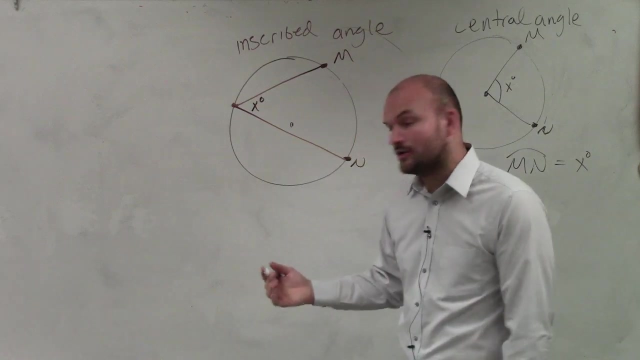 as well as the two endpoints. All right, Now this is going to create some different measurements. We understood that a central angle, the measure of the arc of the central angle, was equal to that angle Right. However, when I'm looking at X degrees for an inscribed angle, 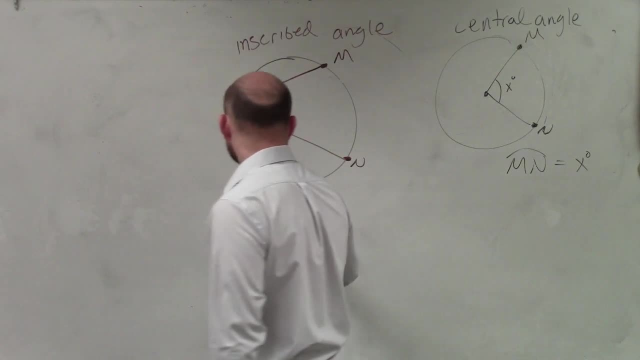 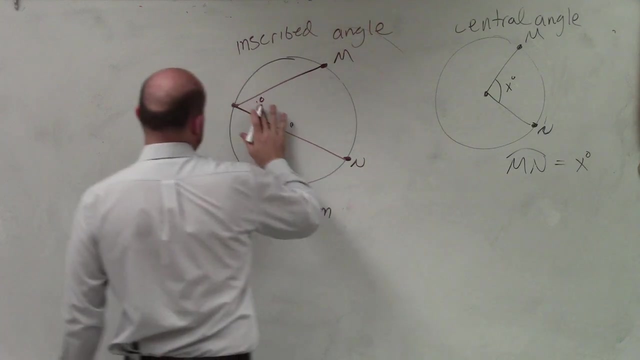 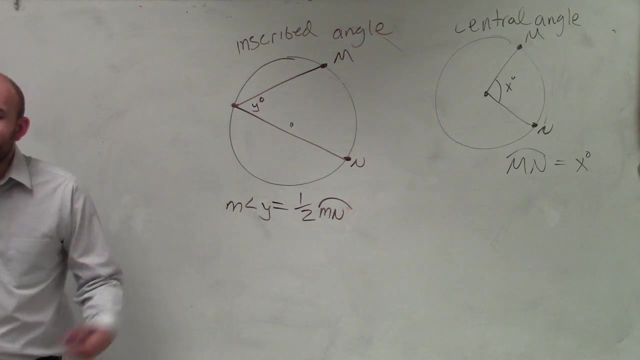 the measure of angle X is equal to one half the measure of my arc m n. Alex, let's call this, let's do a different value, Let's do this Y. Okay, it's actually one half of the measurement. So let's look at this. If here is m to n, this measurement is X. 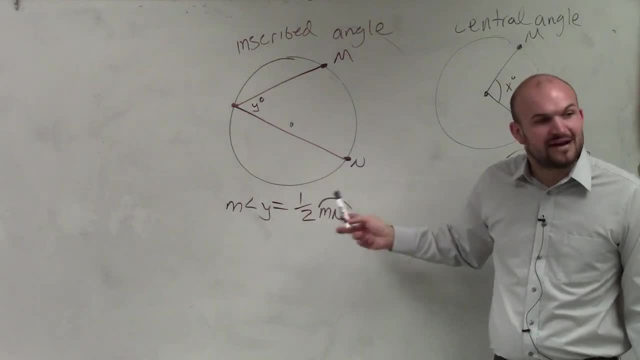 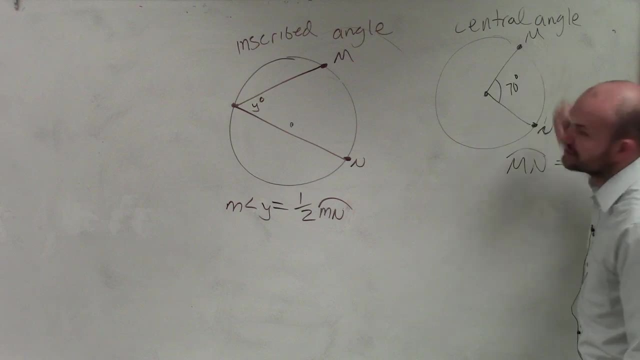 Now the inscribed angle is one half of that value. Okay, So let's put it into perspective. Let's say this is 70 degrees And I say: well then, what is this measurement? If that's 70 degrees, then here's the central angle.